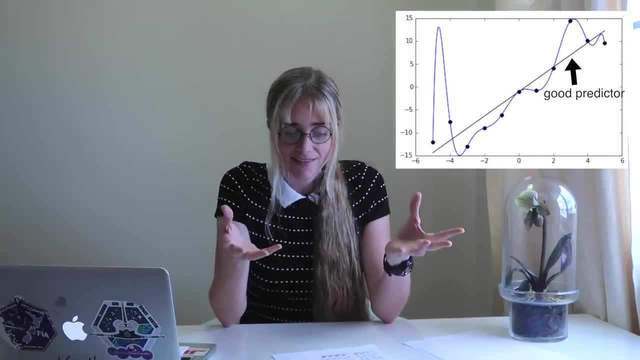 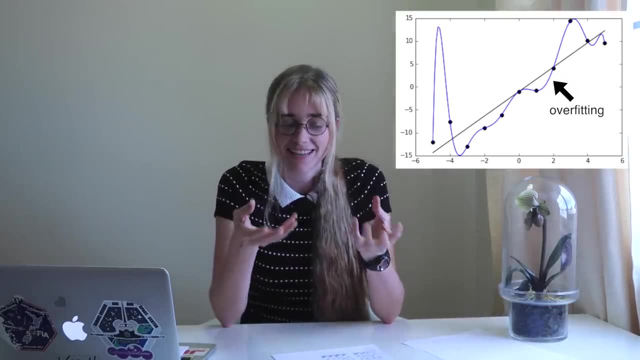 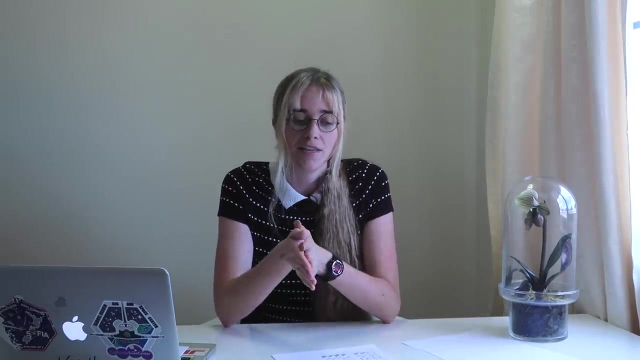 fitting overly complicated patterns to the data which you know, model every single data point and capture all of the noise and random data points as well, not just the general trend of the data, which can be, you know, a genuine problem to have if you're working in, say, machine learning or 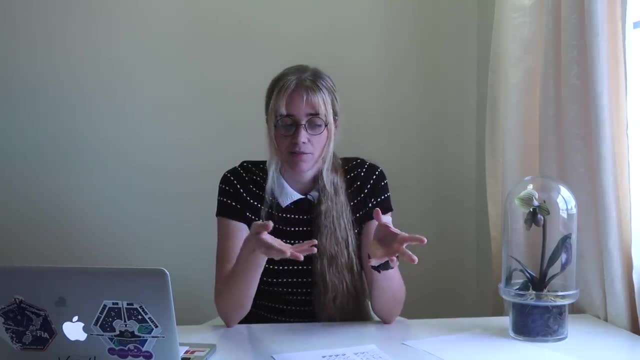 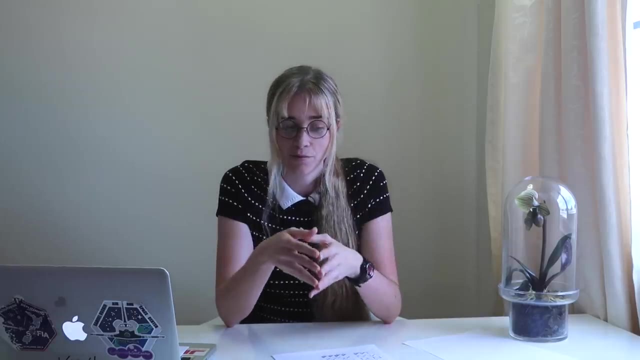 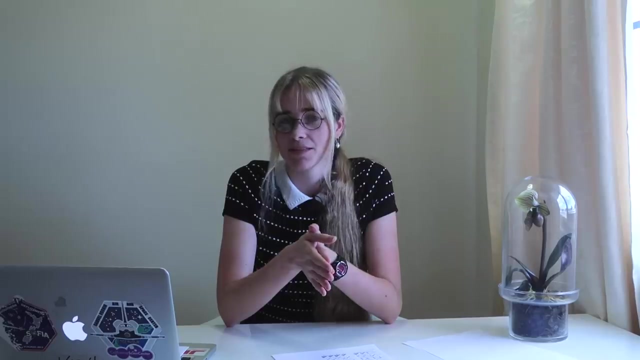 something like that you know, or just trying to predict anything. You actually lose your predictive powers if you start to overfit your data or model it too closely. Back before we knew that the earth and planets orbited around the sun, we had some models, such as the Ptolemy model that earth was at the center of the solar system, and some of these. 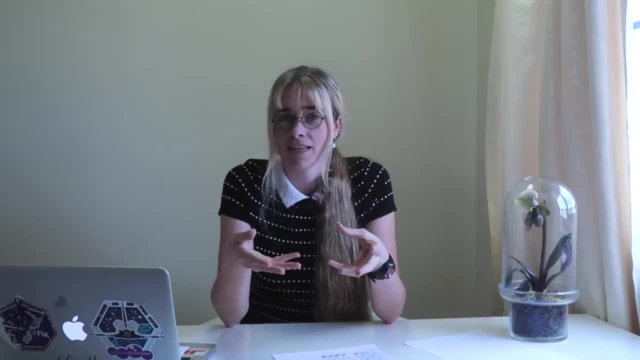 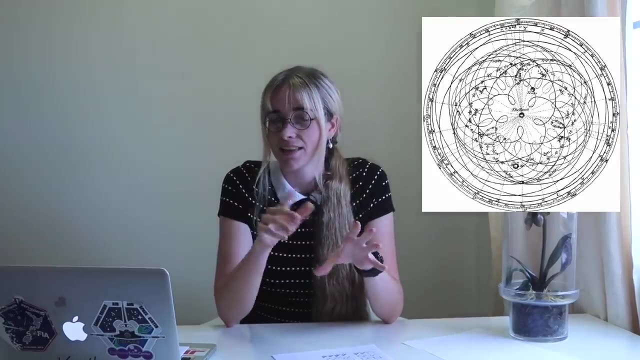 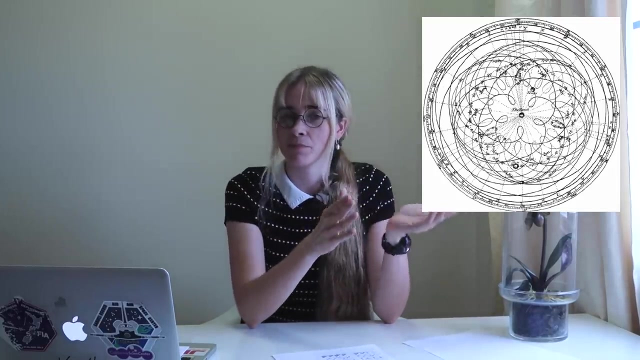 scientists came up with more and more intricate and complicated models to try and explain every single you know data point, A point they could find. they had to come up with elaborate you know circles and loops that the planets were following, which would explain why they appeared to be moving back and forwards. 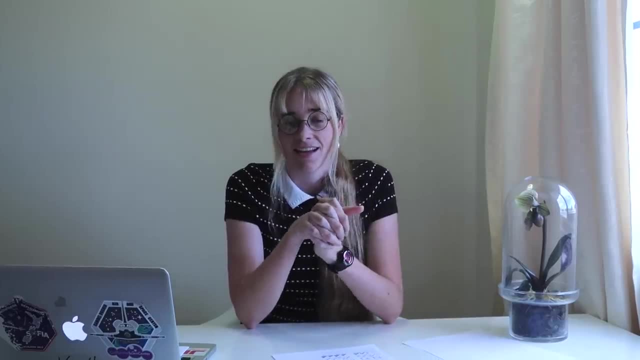 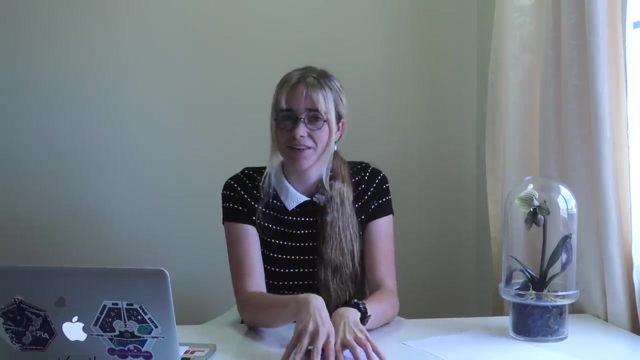 in the sky if they were orbiting the earth. I think it got to a point where this model was just so complicated, trying to explain everything in the wrong way, that ultimately it was better just to adopt a new model that made more sense. This video is filmed on the 31st of July, which is Harry. 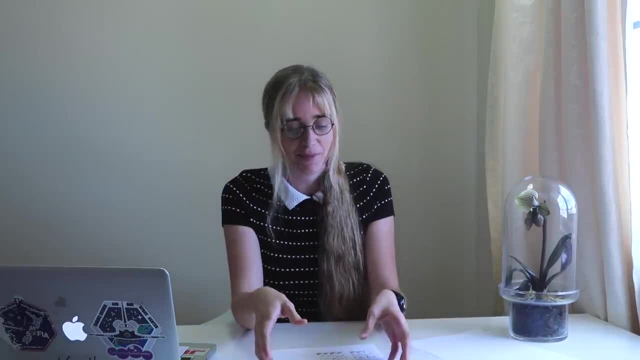 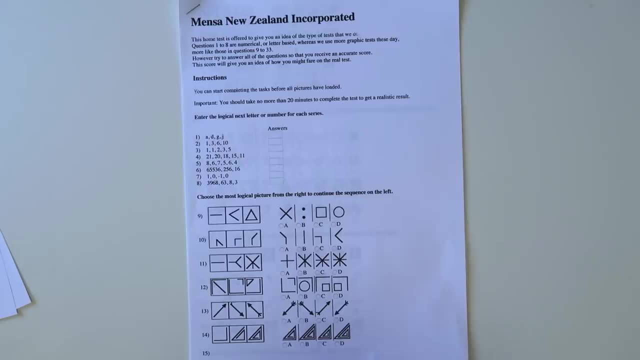 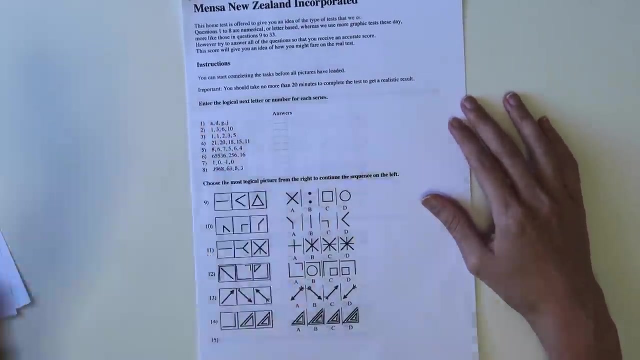 Potter's birthday, so these glasses are a reference to that, but also, perhaps they will give me the necessary IQ points that I need to answer some of these. So here's the exam, and if you've seen my previous video, this will be familiar to you. Now let's just start with looking at the very first. 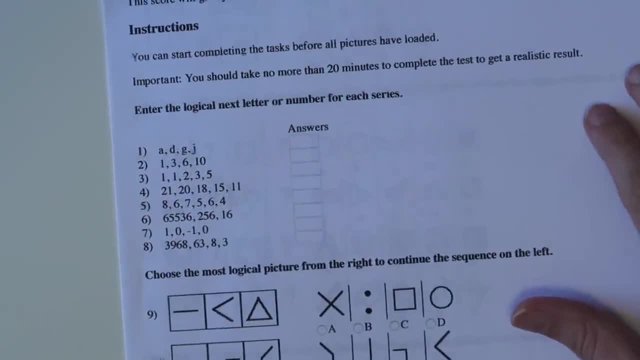 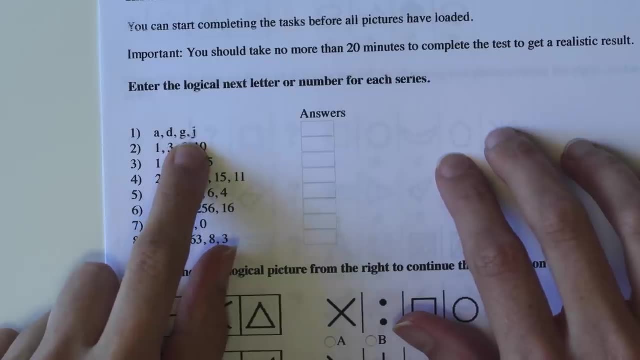 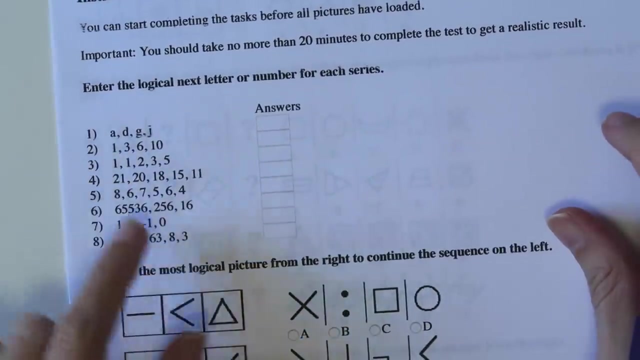 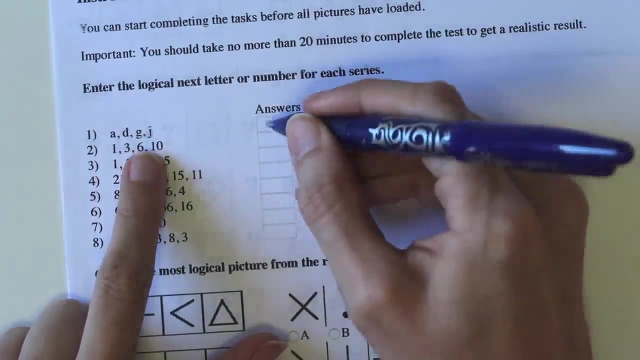 question here Now. the first one is asking us to complete the next in the pattern or in the series now the low IQ or average IQ. way to answer this would be to say that there are two letters missing between each letter here and the answer given in the answers is M, but I thoroughly disagree with. 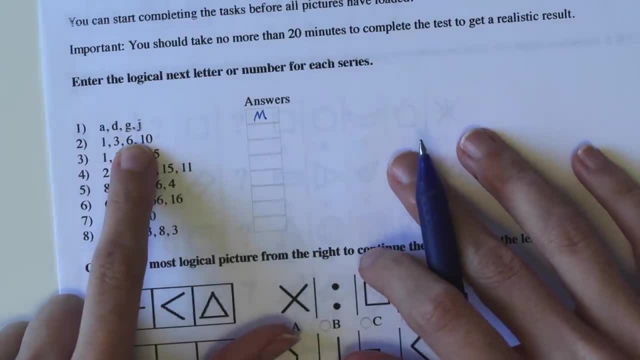 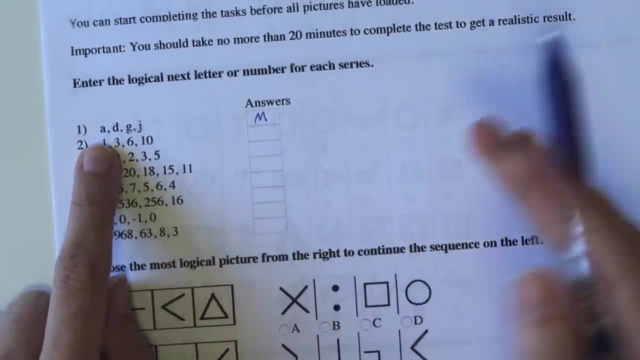 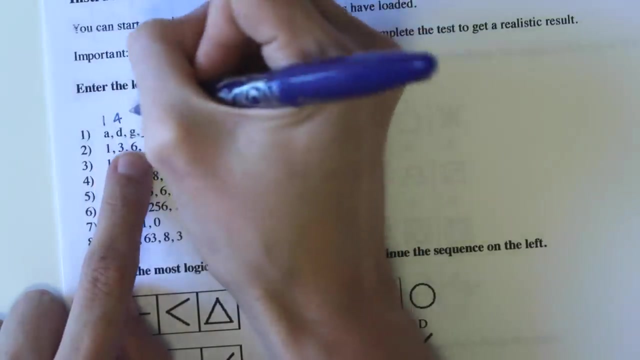 that, seeing as we can do this a much better way, So what we could do is naturally assign each of our letters to their numeral in the alphabet. So A would give us one, D would correspond to four, G to seven and J to ten. Our sequence is now: 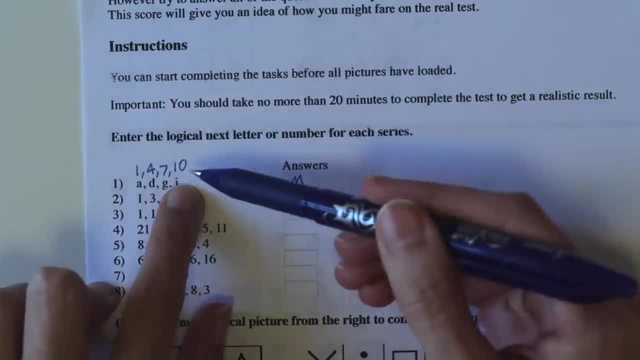 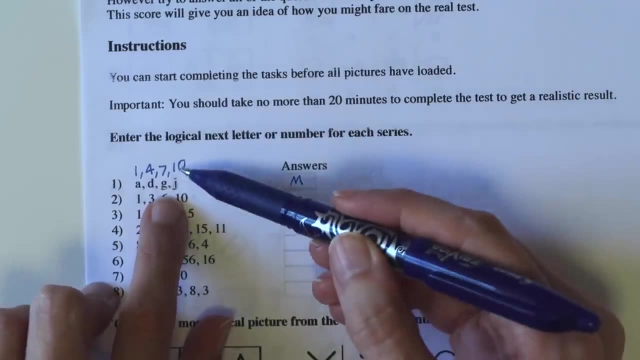 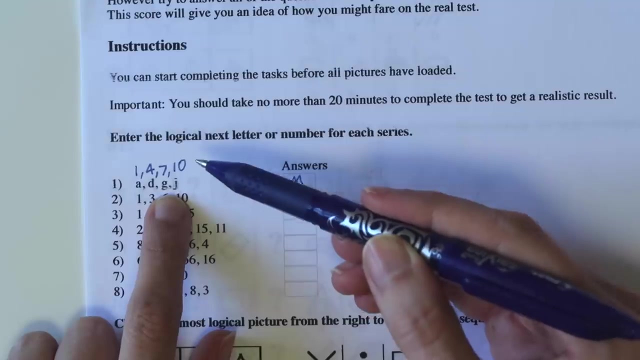 one, four, seven, ten. If we can find the next number in this series, translate it back into a letter. we will have an answer. So what are we going to do to find the next number in this series? Well, I'm going to do the thing that I think would be natural and that's to fit a polynomial. 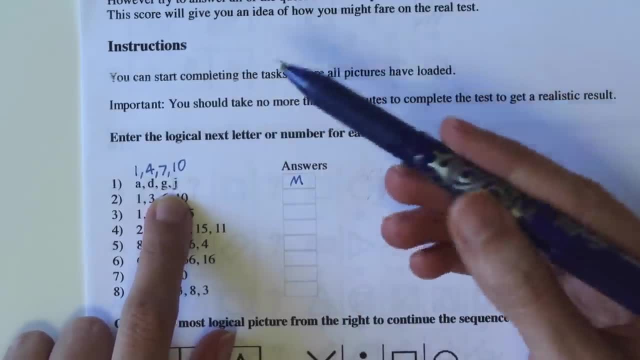 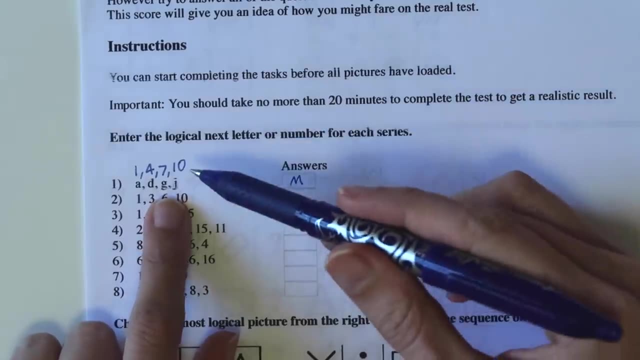 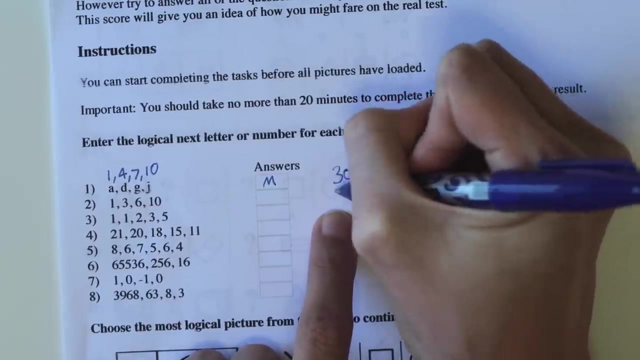 to these numbers. here. You know you can have polynomials of increasing degree to model basically any sequence you want. So I'm going to model this with a fourth degree polynomial which is as follows: 301 over 24, x to the four minus one five. sorry, 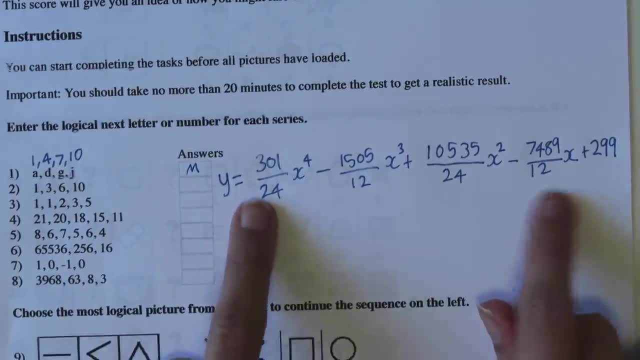 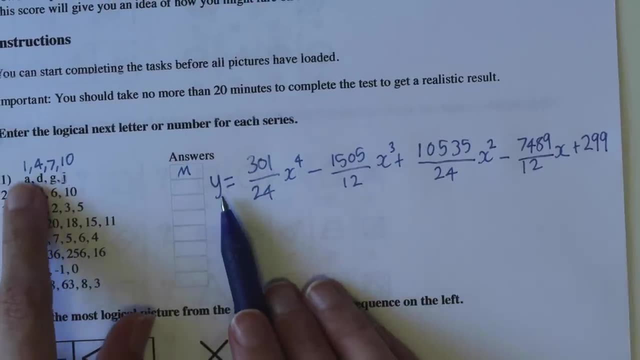 and there's my polynomial. there You can check my working if you wish to. If we plug in an x value of one, we will get a y value of one. If we plug in x is equal to two, we will get four. x is equal. 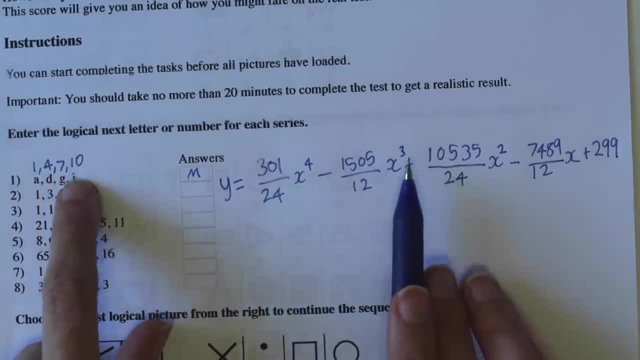 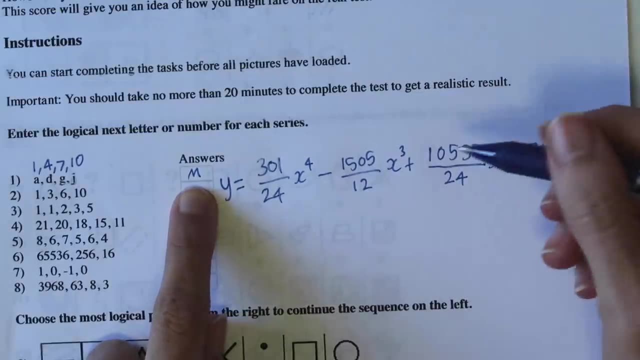 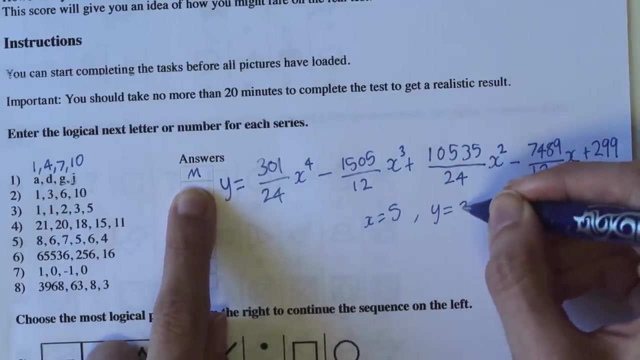 to three, we will get seven. x is equal to four, we'll get ten, and x is equal to five, which is really what we're trying to generate here. our fifth number in the series- Well, x is equal to five- would give us a y value of 314.. I quite like that because it's, you know, an approximation. 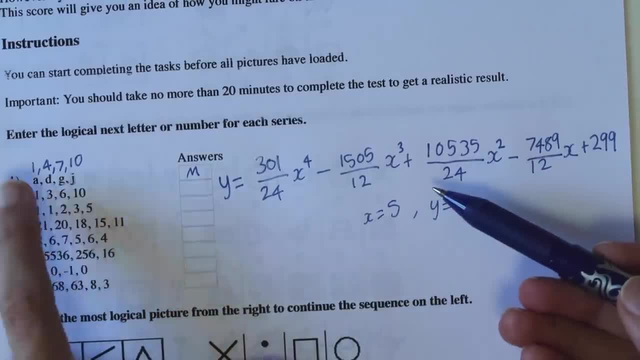 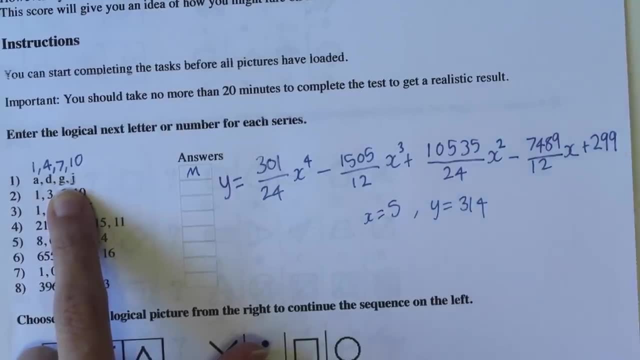 of pi. Now, the only problem is translating it back to a letter. Well, there's not 314 letters in the alphabet. there are, however, 26 letters in the alphabet. so if we do 314 mod 26, we will get an answer of two. 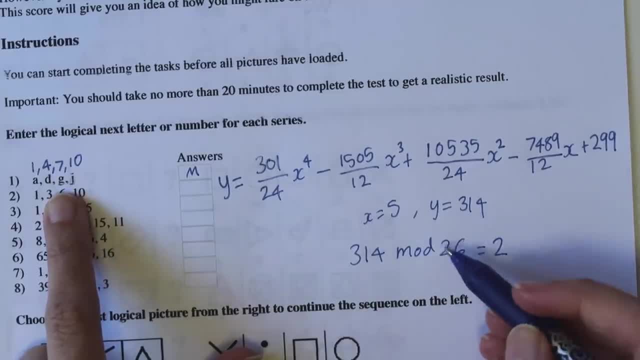 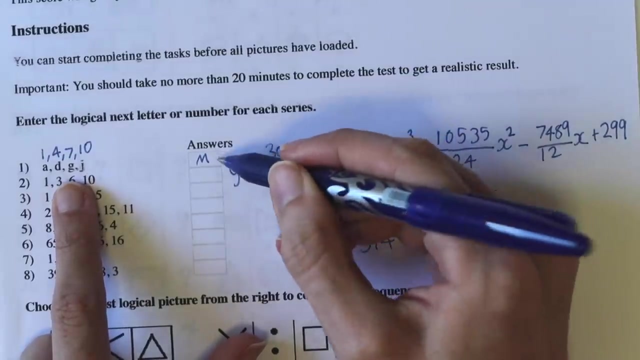 Okay, I'm sure you know how mod works. It's basically the remainder. if we were to divide it by 26. We've got a mod of two which would correspond to a letter b, and now that would be my final answer to the question. It does not agree with the answer given by the answers. 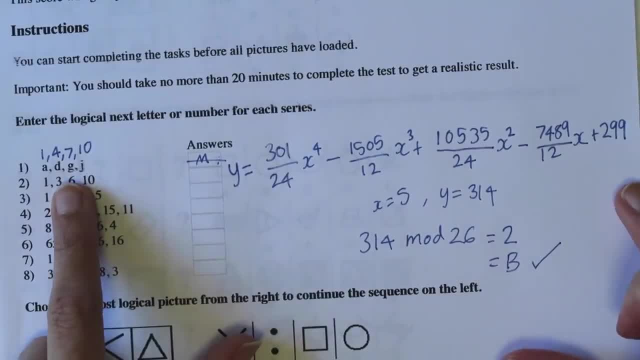 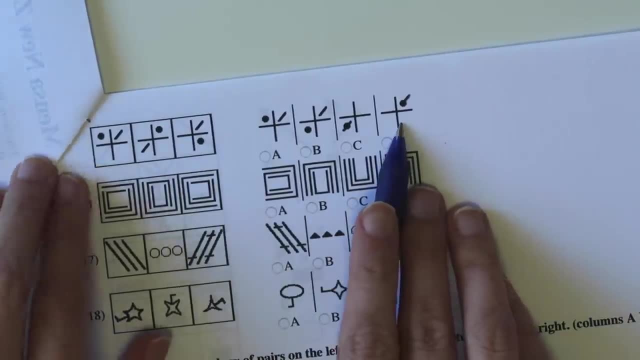 but I think there is nothing wrong with the way I've got it and it is perfectly valid. So, moving on, The next one that I'd like to try is number 15.. It's one of these visual ones. I've watched a few episodes of Rick and Morty before I filmed. 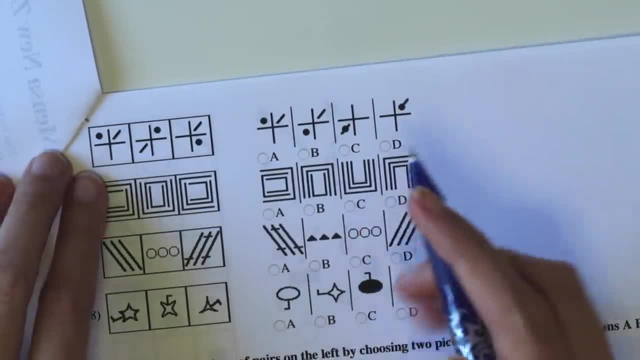 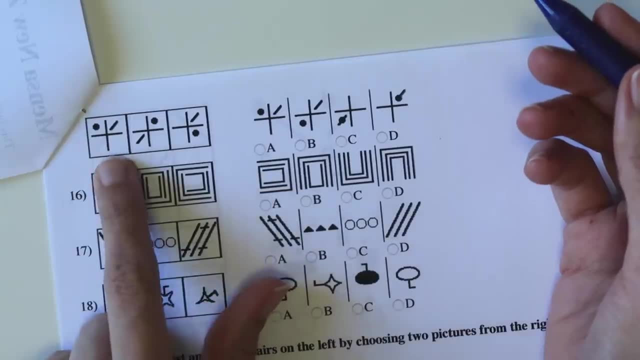 this video, so I should be fine with coming up with something Now for the sake of it. I will give you what the answer says. are the correct answers here? So we're again finding the next one in the series. We've got one, two, three Answers. say that number c is the correct answer. 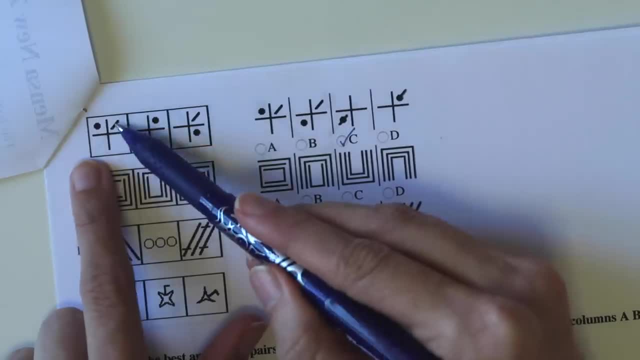 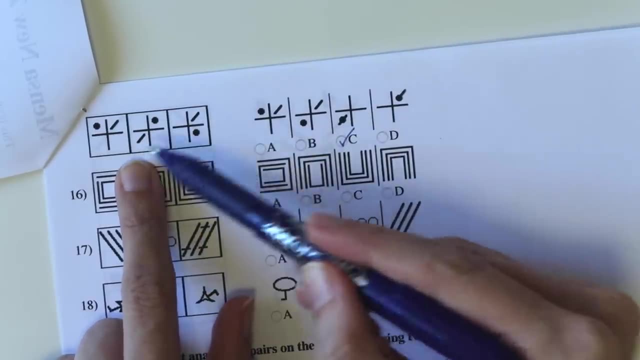 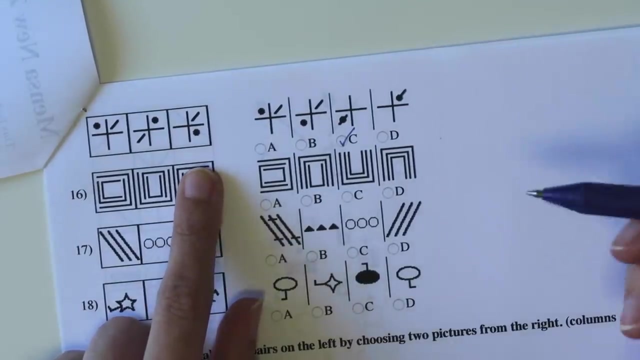 for what comes next. and they say this is true because the dash oscillates between these diagonal faces, so it would oscillate back to here and the dot moves around clockwise, so it would meet the dash there. I mean you could do that or you could do my method. Now there's a little bit of setup. 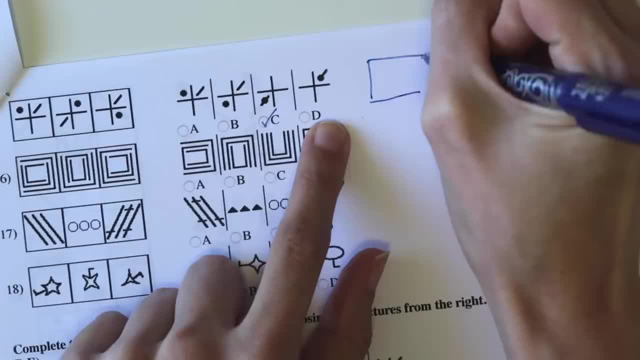 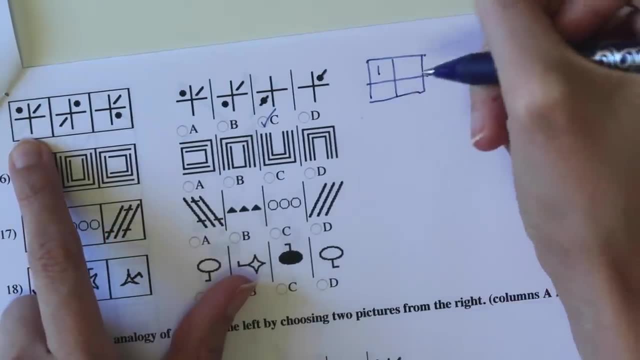 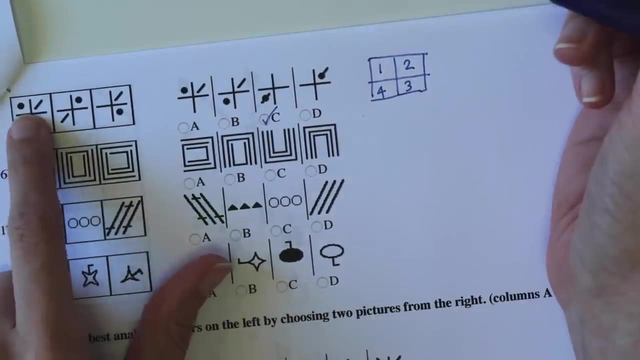 for my method. but essentially, when I look at a square like the one given, I imagine it in a point system where being in this spot here would give you one point, here would give you two, three. and now let's have a look at the behavior of the dot in the first three elements. So in the first one. 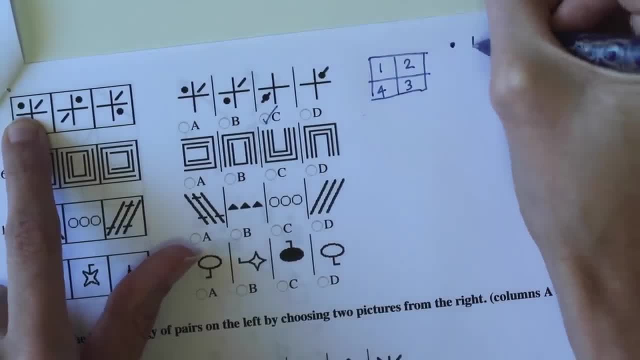 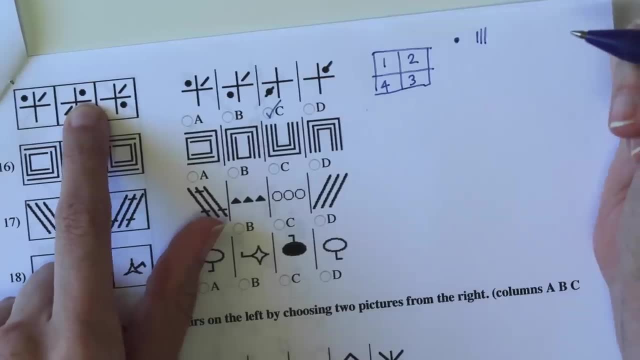 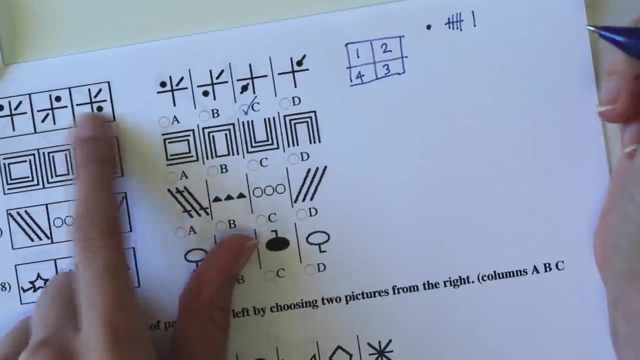 it's in position one, The dot has accumulated one point. In the second one it moves across to spot two. It's now got an additional two points, and in this third one it's moved down to have an additional three points: One, two, three. At the end of this the dot is on a tally of six points. 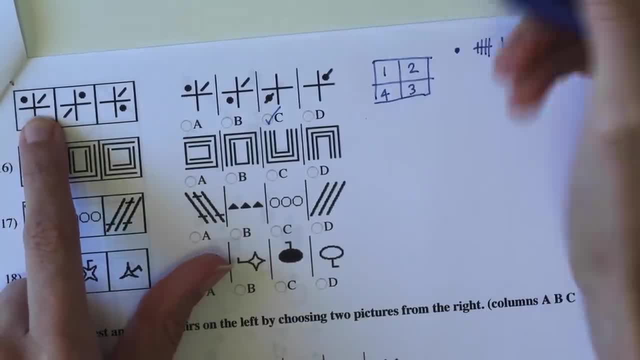 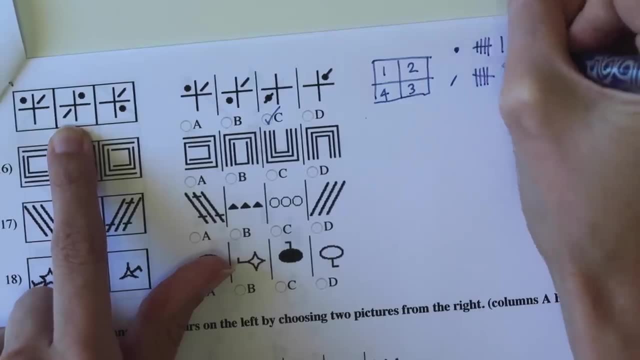 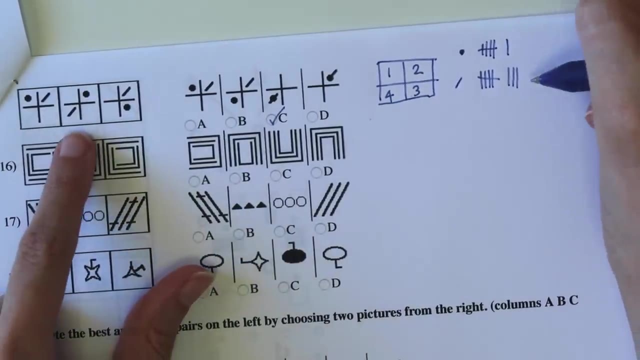 Now let's look at the behavior. The dash starts off in the two, so it has two, then we can add to that four, and then we can add to that another two. Now you know, we've got a tally of points for both of them, but what are we going to do with that? Well, the only logical thing to do with that would to be to 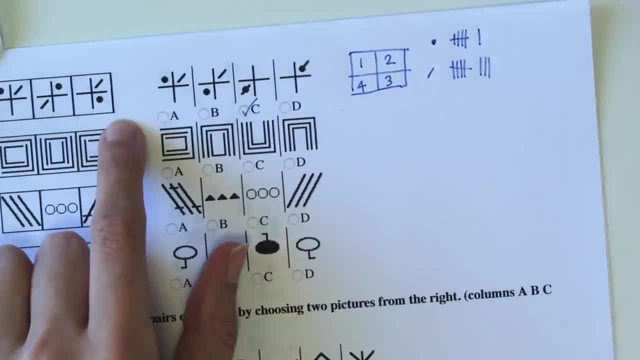 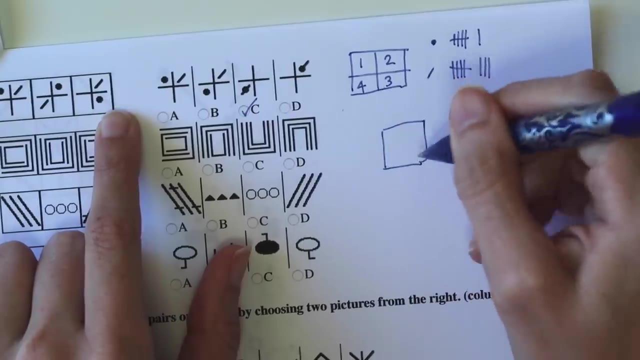 think, okay, we've got, you know, one more element in this series, and wouldn't it be great if, with that one last iteration, we could make the points for both of the shapes equal. Now, there are a couple of ways that this could happen, actually, and I'll draw the two possible options for the fourth. 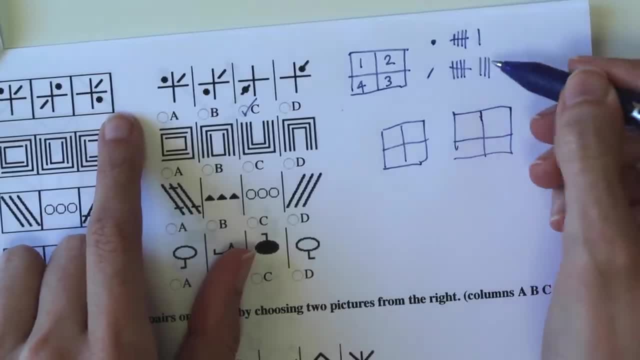 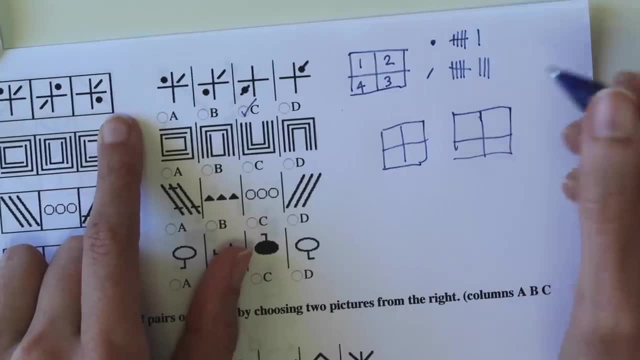 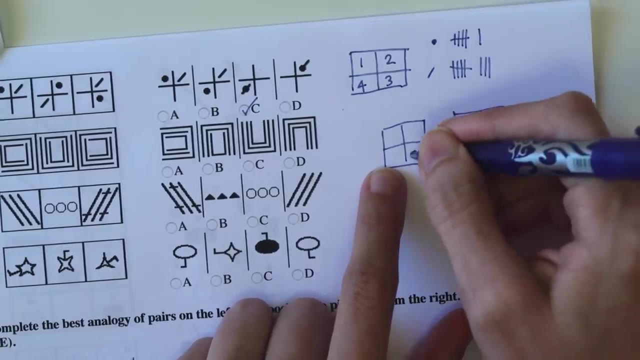 item in the in the series. So the dot and the dash. well, we've got six, and we've got eight. Well, we could imagine that they could go on to both equal nine, where the dot could gain an additional three, so it would have to be here, and the dash would gain an additional one, so it would be here. 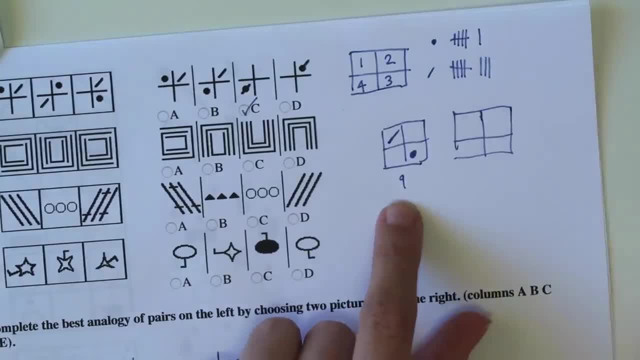 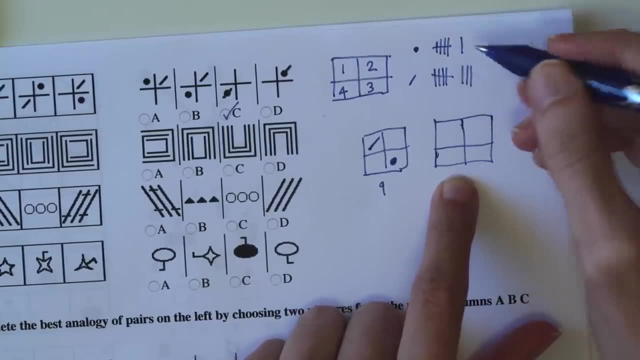 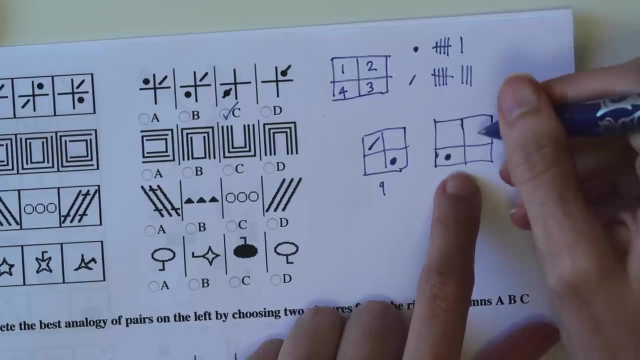 I guess that would be one option where the tally would come to a total of nine. Our other option is to bring the tally both to a total of ten. so the dot would have to gain an additional four placing it here. The dash would have to gain an additional two placing it here. 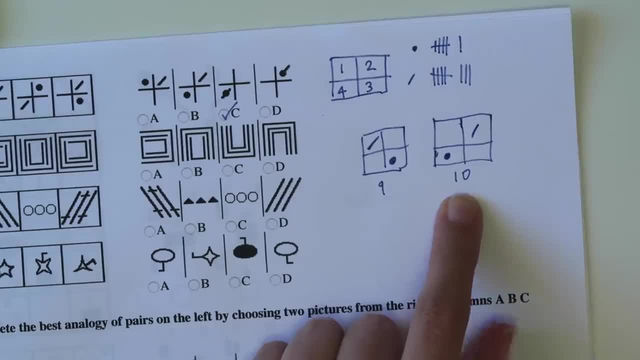 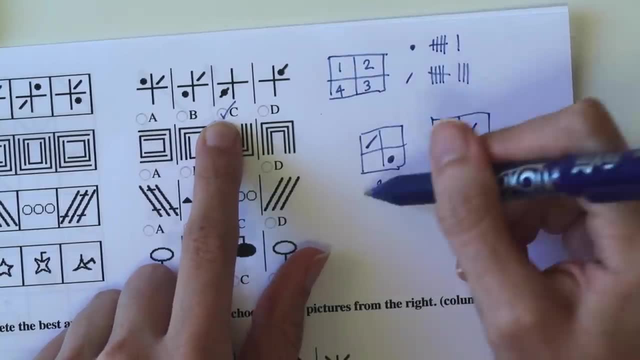 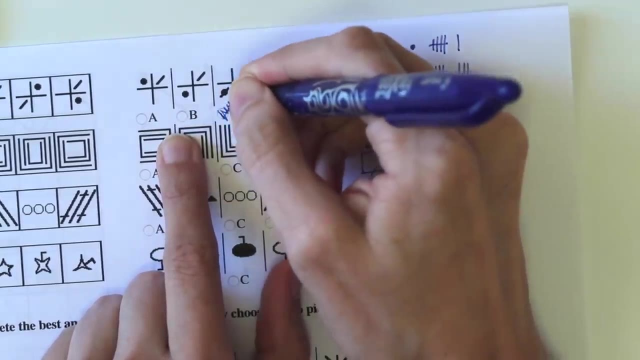 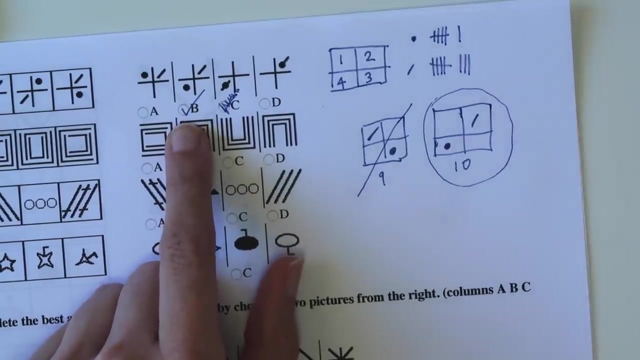 All right, so that gives us both a total of ten. If we look up to our possible answers, to pick from this option here does not appear as an option, but this option here does. so I would say that my better and more correct answer would be B. I say the phrase more correct, but of course I mean that they both could be correct. 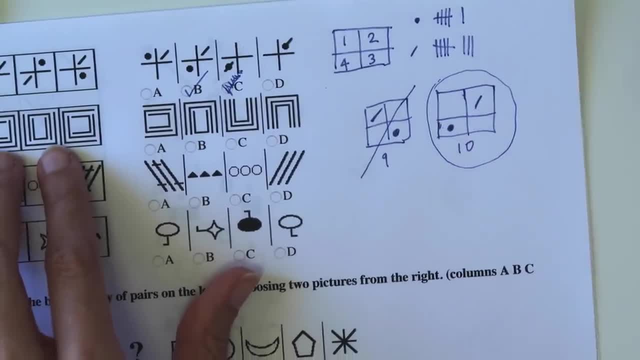 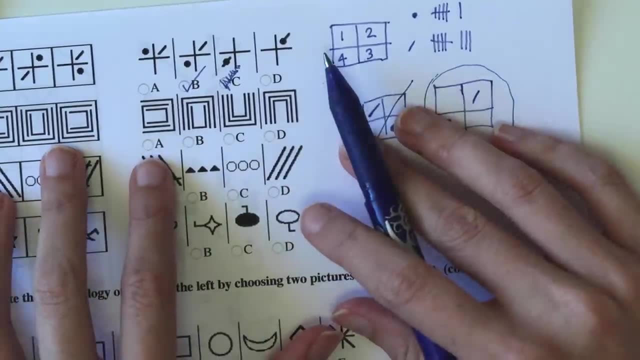 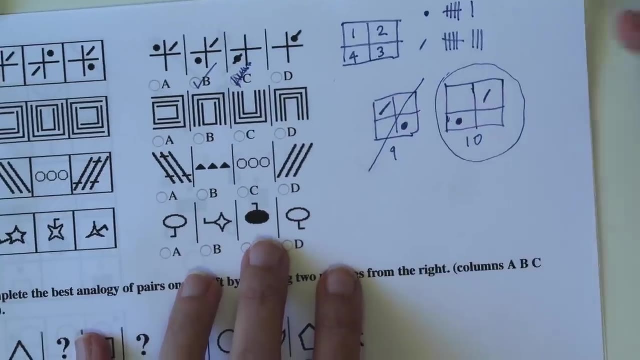 depending on what you're looking for here. If you're looking for a IQ 300 play, you know, maybe that's what I've shown You. but if you're looking for how to score well on this test being marked by whoever is marking it, then you'll have to try and simplify your reasoning down to give an answer of C. 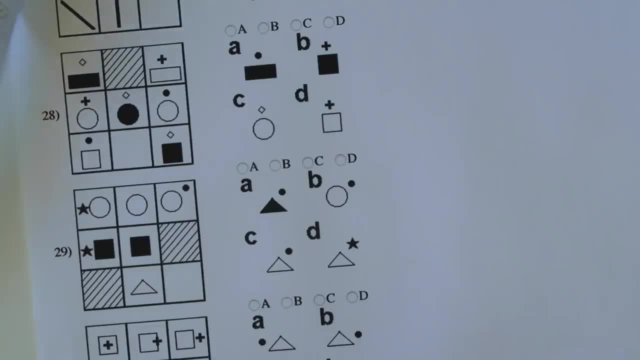 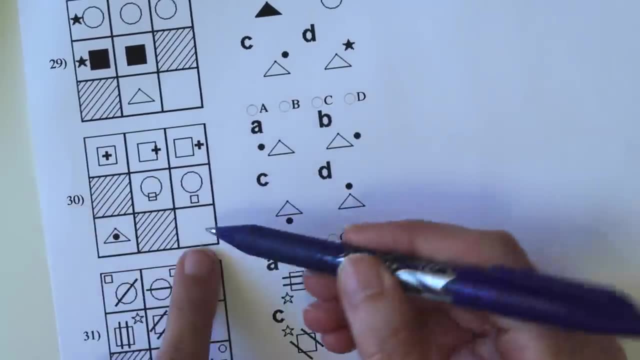 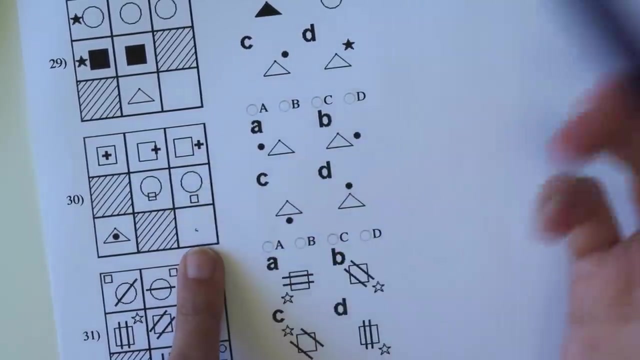 I'll try out one last one on the last page. Okay, so number 30 is a little bit different from what we've done already. We are wanting to find out what shape would go in this box here. so there's obviously some pattern things are following and to make it a little, 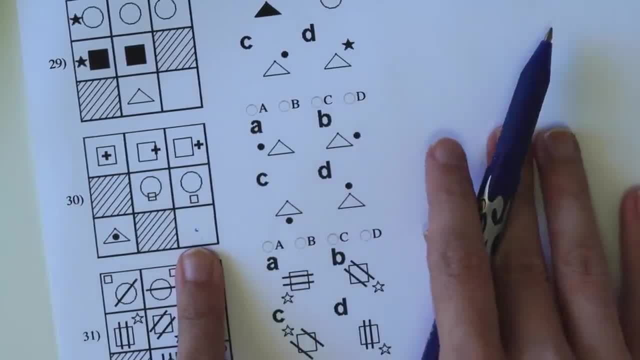 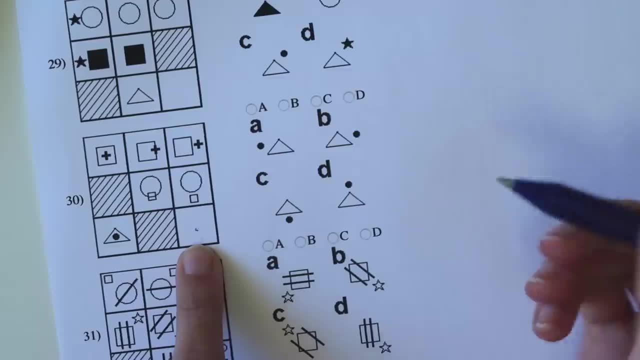 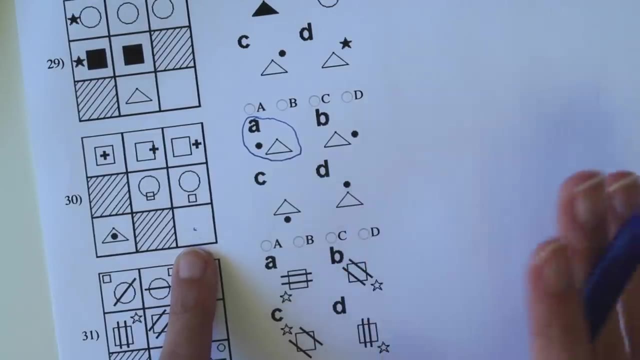 tricky. they've blocked out these two squares, so we can't see what was going on there, but we can still work out the pattern, fine enough. Now, a quick glance at the answers do say that A is the expected answer for this, so let's see if we agree with them Now. first of all, I want to find out what is happening between: 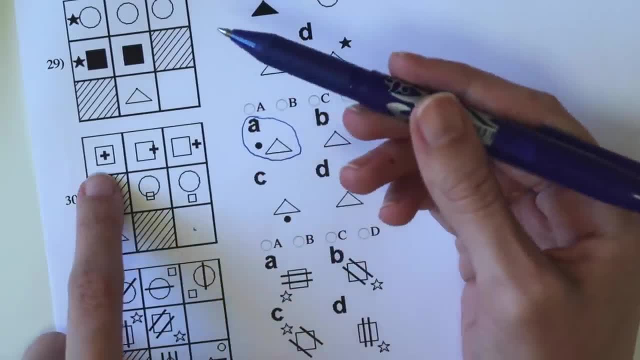 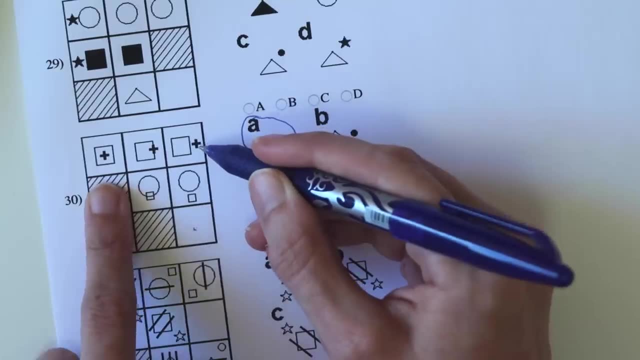 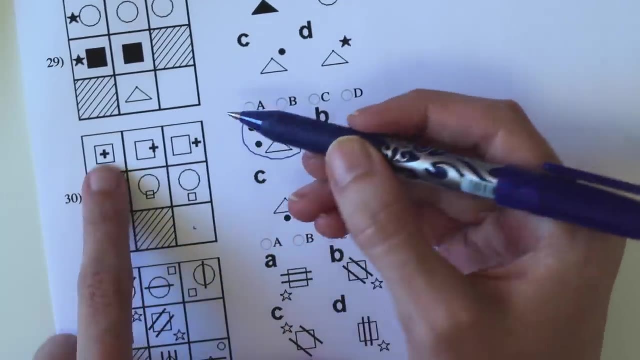 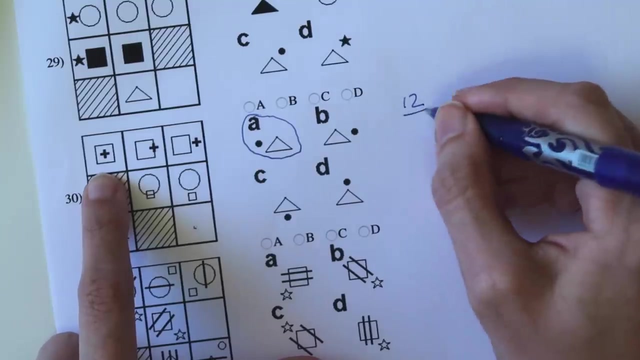 this first line and the second line. so I, just from looking at it, can see a sort of a pattern already. So let's look at the number of sides on the smaller shape and divide it by the number of sides on the larger shape. Well, what we would get is that the cross has 12 sides. the box has four sides. 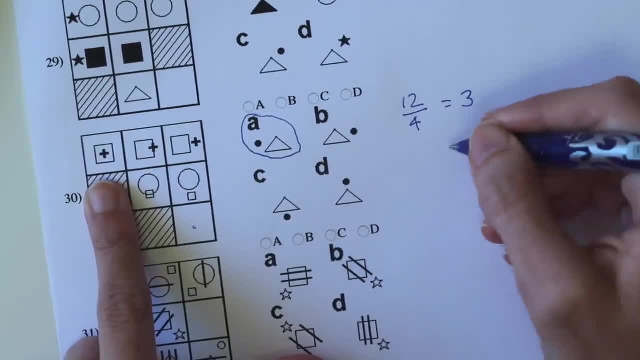 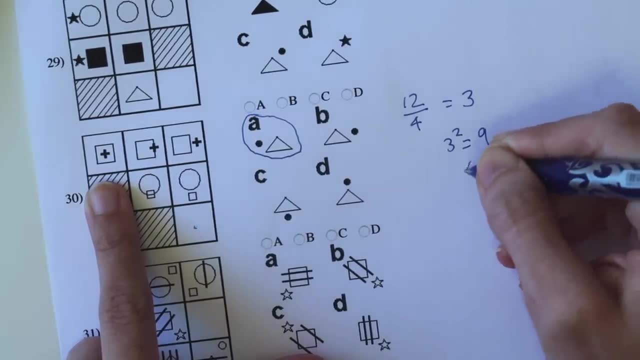 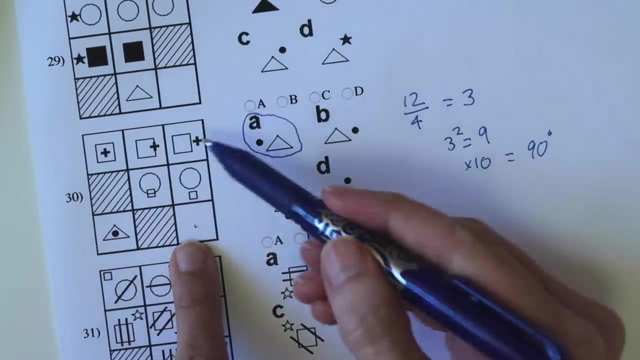 that division would give us 3, but if we were to square 3, we would get 9, and if we were to times that by 10, we would get 90 degrees, because that is how much it rotates in terms of where it's flying off to. 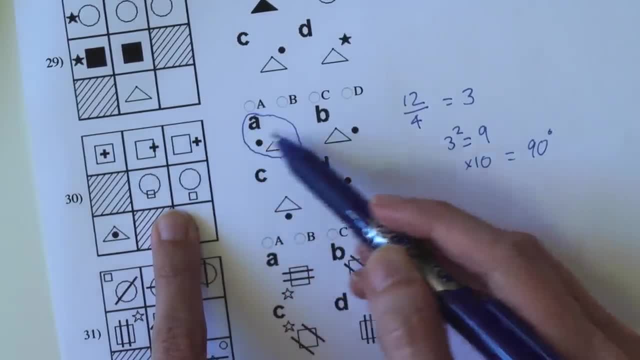 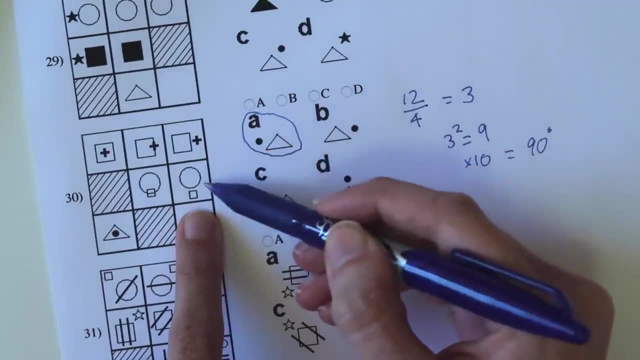 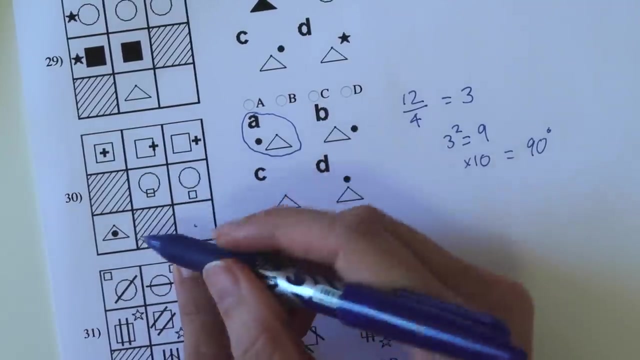 between this line and this line. Here it flies out to the right. here this little box appears to be flying down, you know, downwards. so that's a difference of 90 degrees. If we do the same logic, I think we can find out what kind of rotation this box would undergo when it turns into a dot. 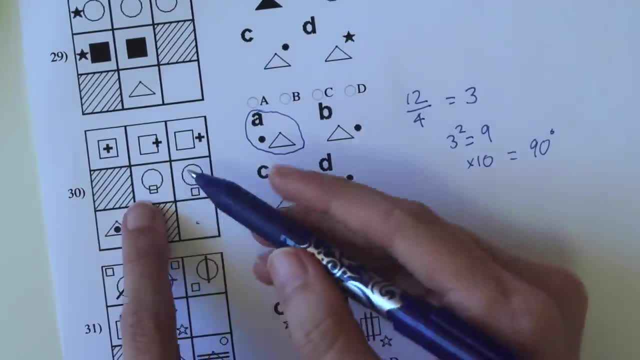 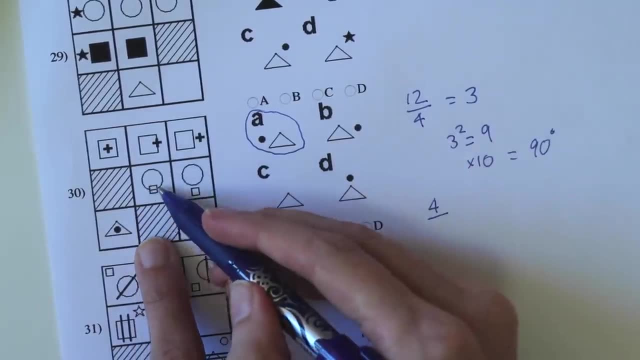 and what angle it would fly off at. Now, if we were to do the same logic, we would get 90 degrees. So let's count the number of sides of the little shape. we have four, so that would be four divided by well, a circle has one side, so that would be four over one. that would be four, four squared. 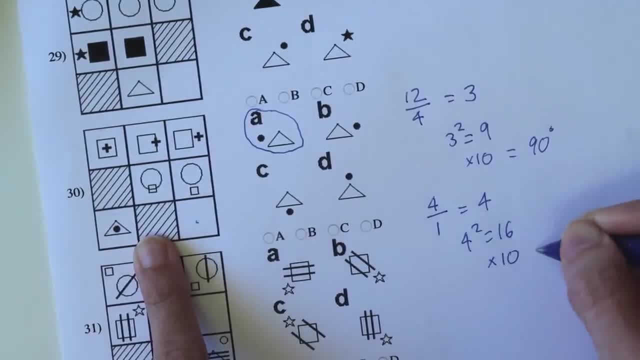 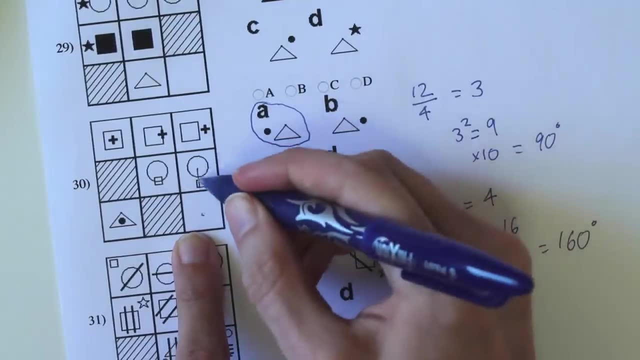 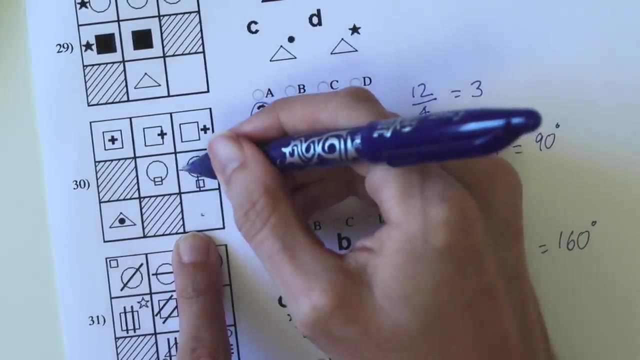 would be 16 times 10 would give us 160 degrees. So if this one is starting from the downwards position, we want to rotate 160 degrees, well, that would be 90, and then we'd have 70 more. We would expect a triangle with a circle flying out. 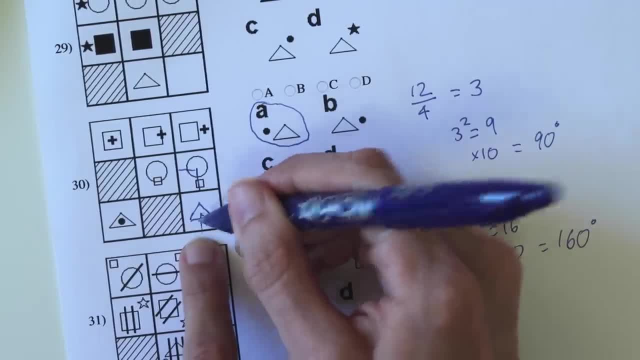 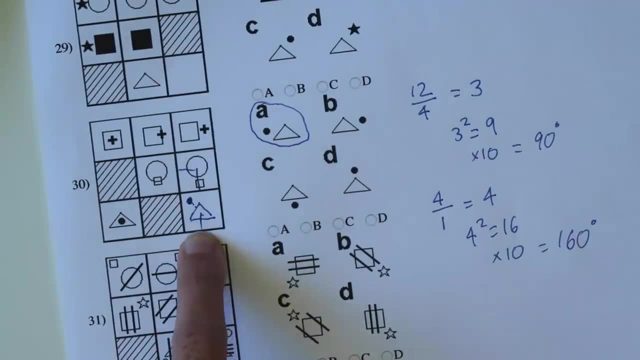 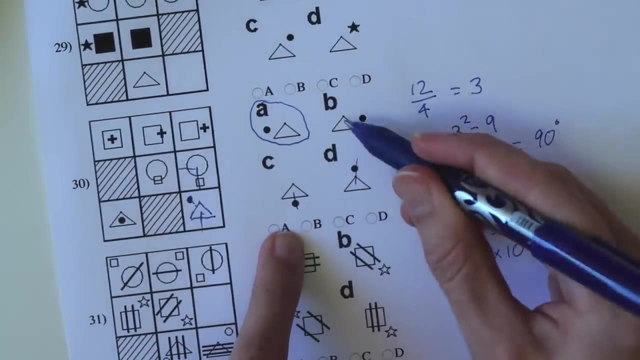 at 160 degrees relative to the base, so I would expect that to be somewhere like there. Now, that doesn't quite perfectly match any of our answers. this one: it flies out to the bottom, to the top, to the right. well, it's definitely none of those. 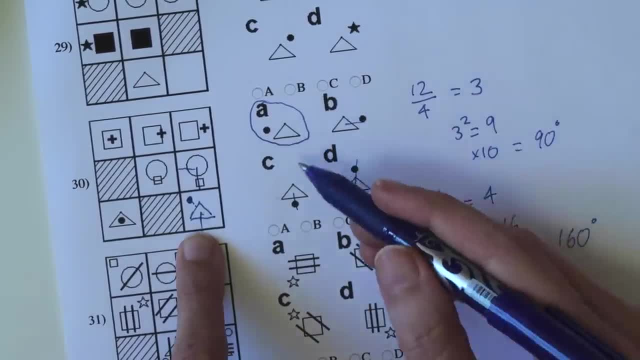 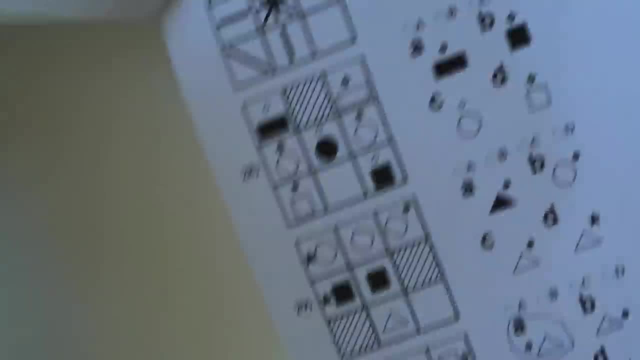 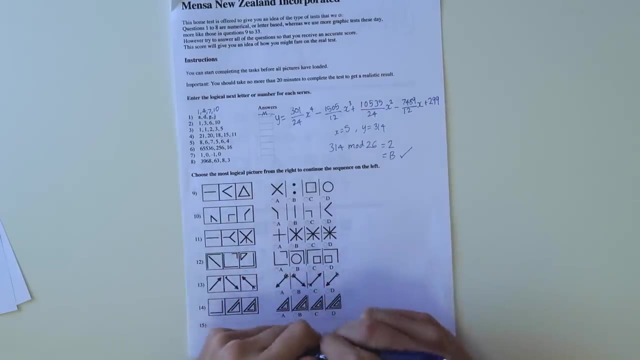 so I would agree that a fits our pattern most precisely, although not exactly. And there you go. I've solved a few problems there and I guess you can try out the rest of them for yourself, if you haven't already, from my last video. So don't take that too seriously. it was really just a bit of fun. 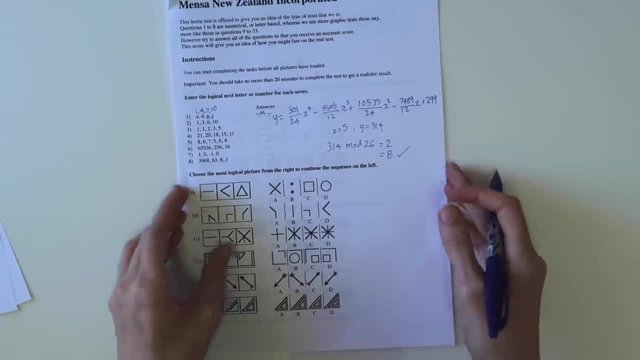 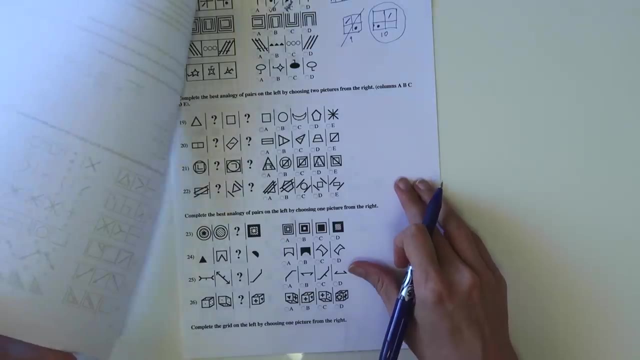 to see if we can fit a model to anything we want to and kind of force our way to any answer possible. I guess there's something to say for, you know, trying to measure intelligence from one set of answers, Whether mine are more intelligent or less intelligent. 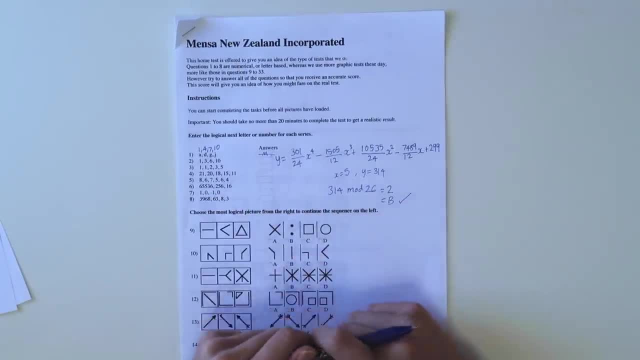 is up to the viewer to decide, but thank you for watching.